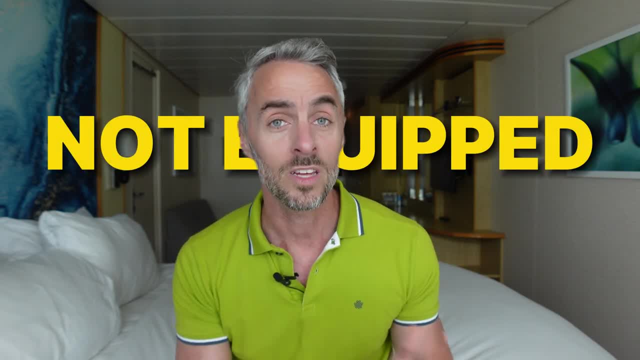 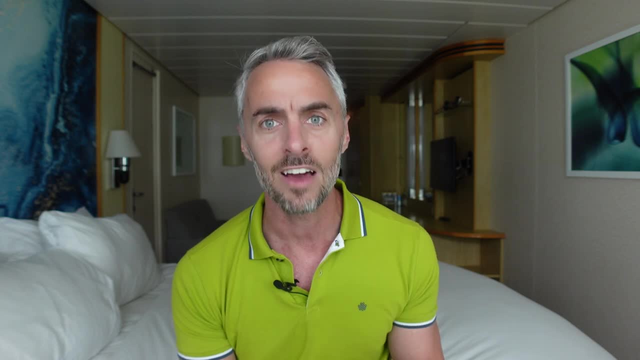 cruise ships there and they've got makeshift terminals but they're not equipped for this. So you are going to find a lot of long lines every single day when you come back to the cruise ship. I think on my last sailing we had five ports. three or four of those had 30 to 45 minutes standing. 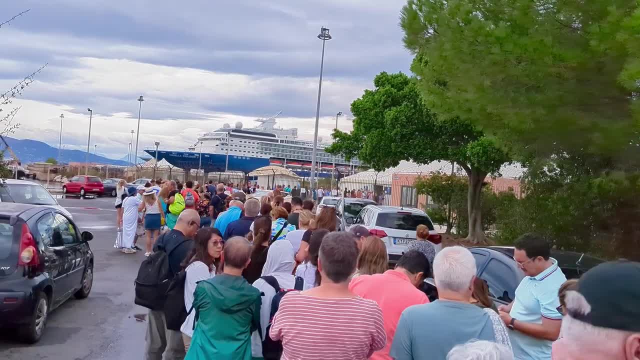 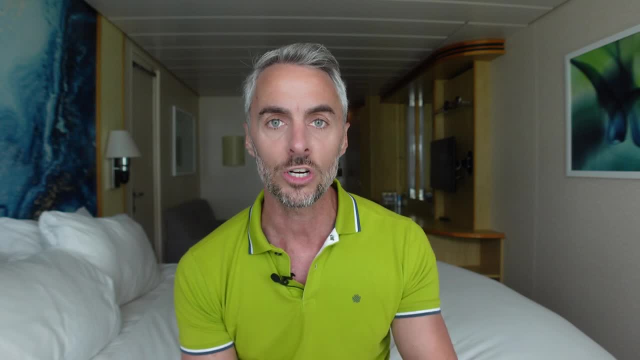 waits to get back onto the ship And there is nowhere to be able to sit And in most cases we were standing outside, for sometimes even in the rain. Luckily they do do the security screening out here at the ports. You don't have to go through that once you get to the ship. 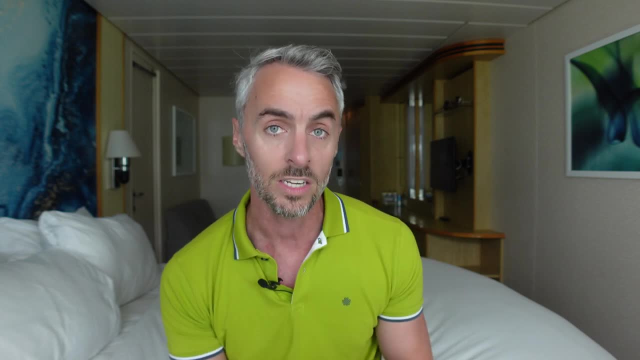 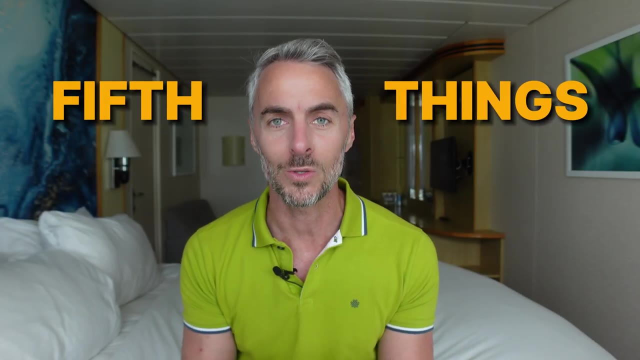 but do expect them to be on your feet for 30 to 45 minutes to get back onto the ship, because everybody's coming back at the exact same time And, with all these cruise lines bringing more people over to the ports, you're going to find that. number four is: there is a ton. 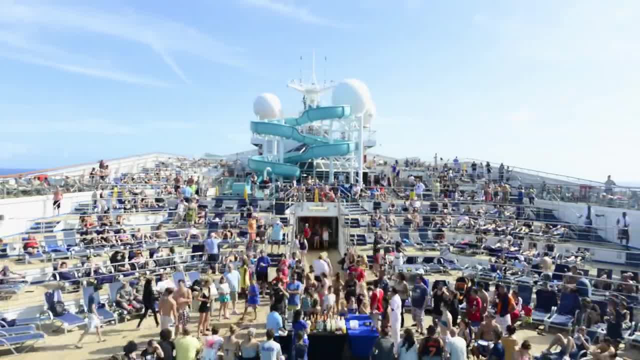 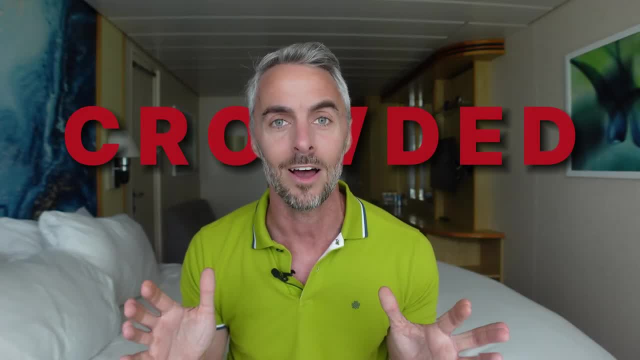 more people in these ports. You thought Nassau was crowded. Nassau is not crowded. Compared to Mykonos midsummer, compared to Santorini or to some of these other ports where you're going to have four or five ships all tendering in, it is going to be exceptionally. 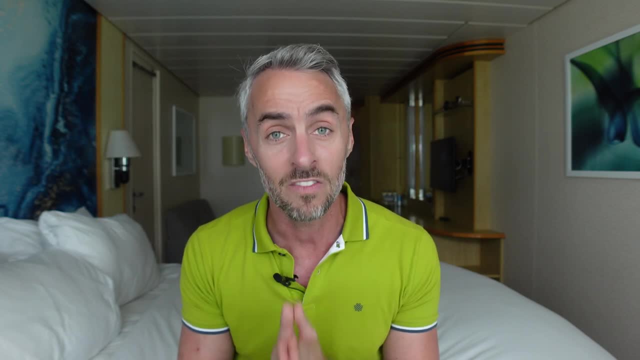 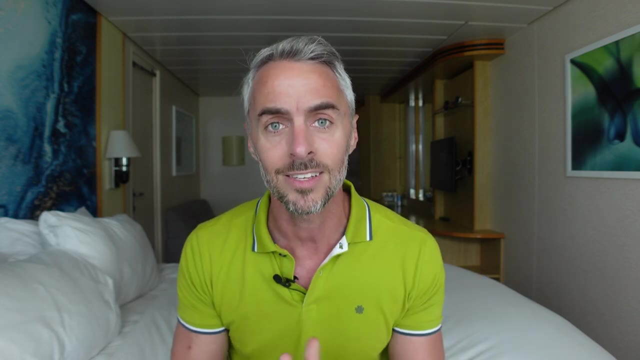 crowded with the normal crowds that they have there, And it's also going to be very hot. But be prepared for all of the people. Just set your mind frame that the beautiful pictures that you see are going to have tons of people. in The sixth one here, and my personal favorite, is, you're going to 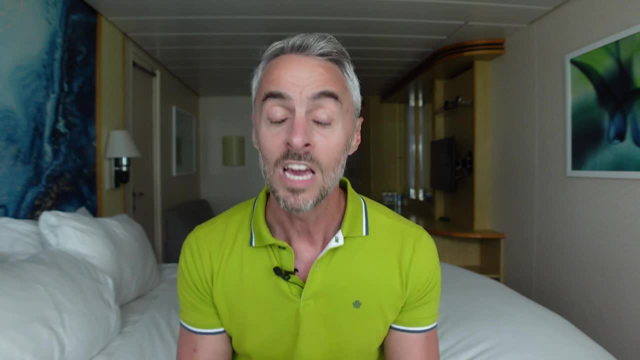 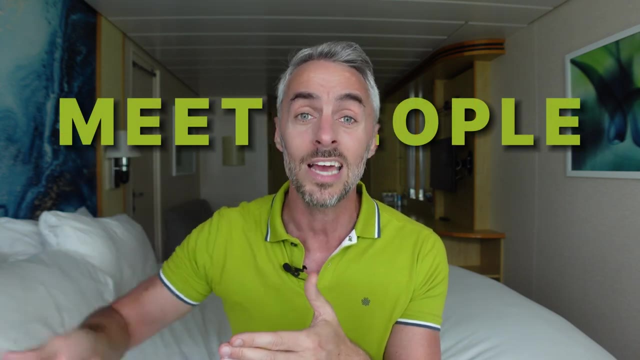 get the opportunity to meet people from all over the world. So the cruise lines, even American cruise lines, because it is in the Mediterranean, you're going to have people flying from Europe, It's super close- Middle East Asia, even South American people want to come over and people from 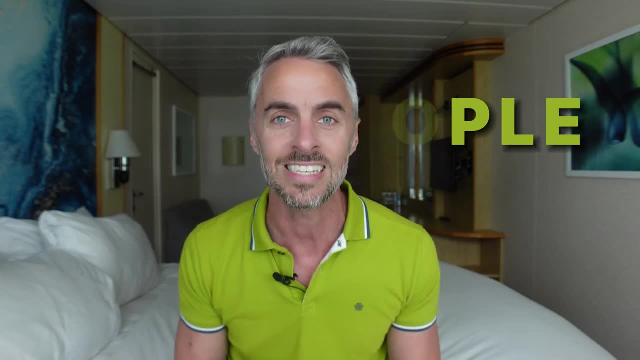 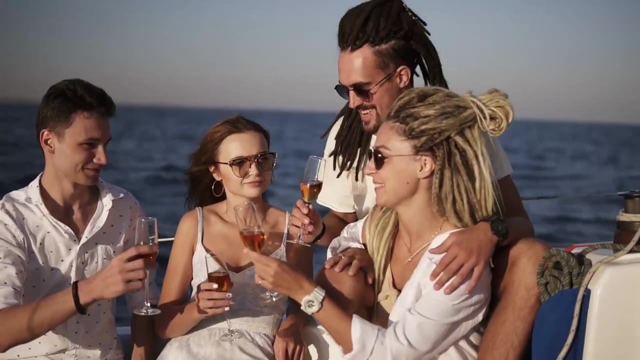 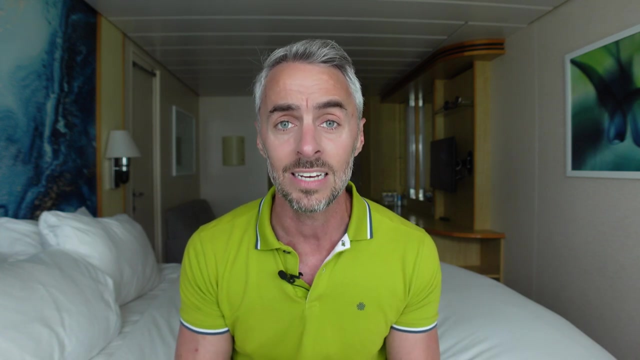 Africa. I met people from all over the world on this sailing and I loved hearing their stories, all the accents. It was a beautiful thing because I can't think of another environment where I had the opportunity to see such a diverse group of people come together and have an amazing 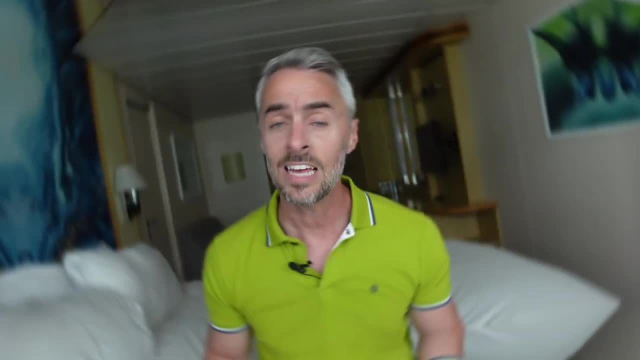 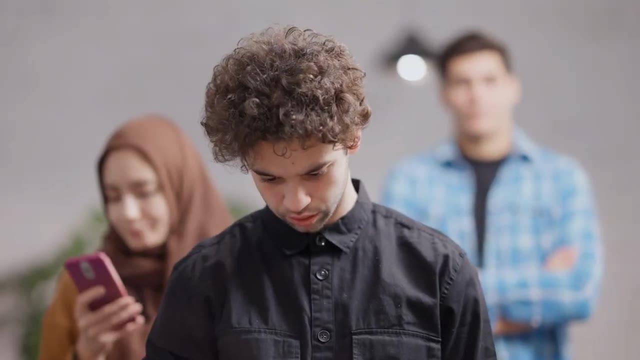 experience as part of a cruise ship community. The seventh one here, and this is probably one that will drive some people a little bit mad- is that you're going to hear the announcements in multiple different languages. So when the cruise line is coming over the loudspeakers, the PA system. 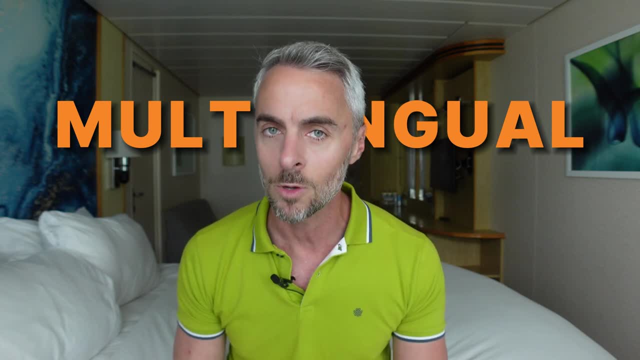 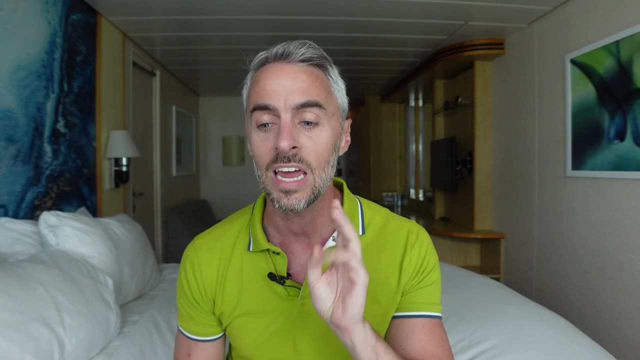 to tell you what's going on or to do a drill. they're going to do it in multiple languages. So, on my personal sailing, it was done in four languages. each time It was done in English, Italian, Spanish and German were the four languages that they did all the announcements. 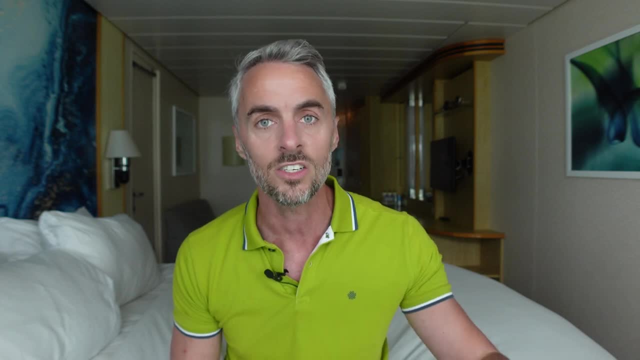 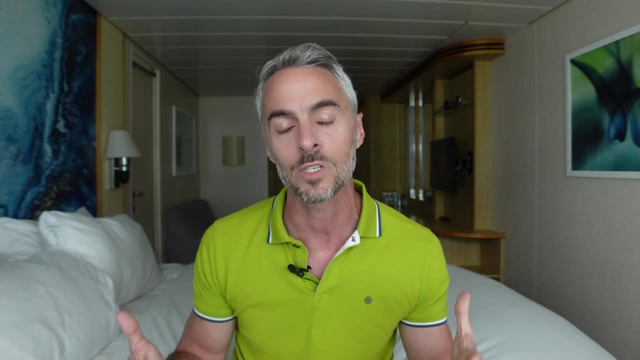 in The announcements are going to be determined based on the percentage of people on that ship. So if there's a lot of Germans on the ship, you're going to find the German language there. If you see another country has a really high percentage, they're going to make it in that language. That is. 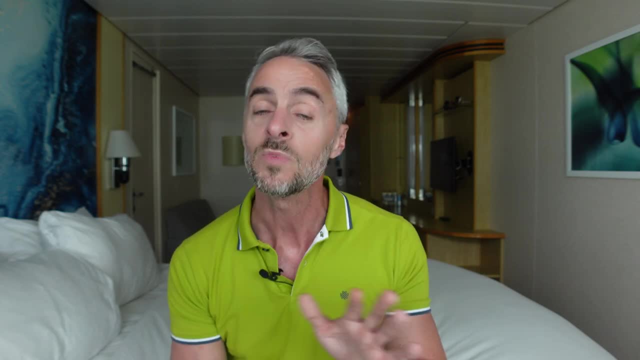 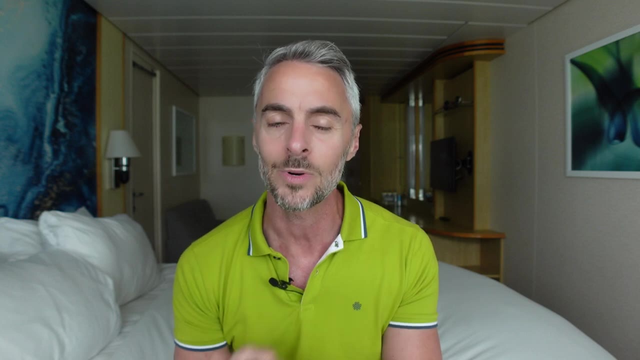 something you don't really see a lot of in the US or Caribbean ports Sailing out of South Florida, England and Spain. that is not uncommon, But then when you add two more to it, that's where it starts to get a little bit different And, honestly, those announcements start to go on. 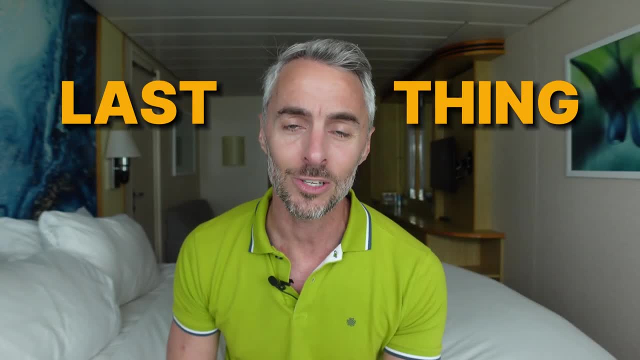 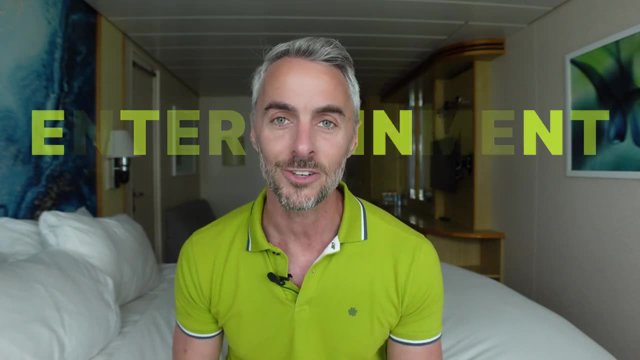 for a little bit longer. And the eighth one- and I think that this is just a smart move for Royal Caribbean to save a little bit of money- is they bring in a lot more international entertainers and headliners to keep us entertained, So they're going to be finding Italian singers. They're 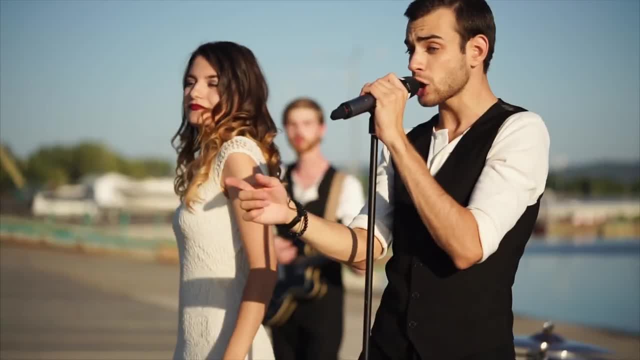 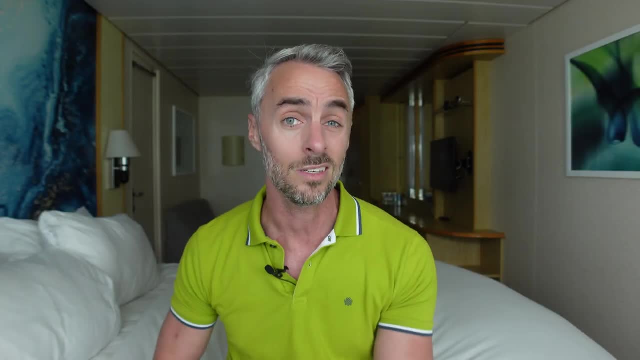 going to find people from Spain, people from the local area, to bring in, And so this means that you're going to have a different variety of entertainers that you might not have seen over in the Caribbean. In the Caribbean, I've seen just about every single juggler that Royal Caribbean. 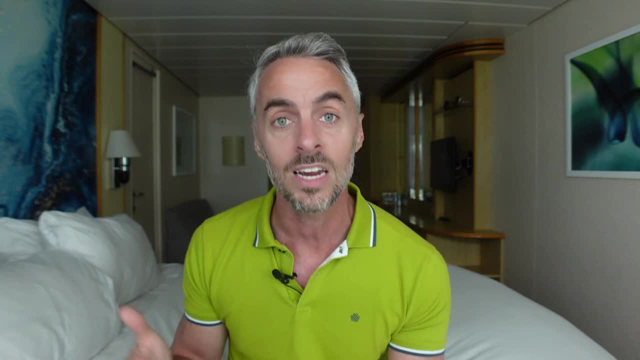 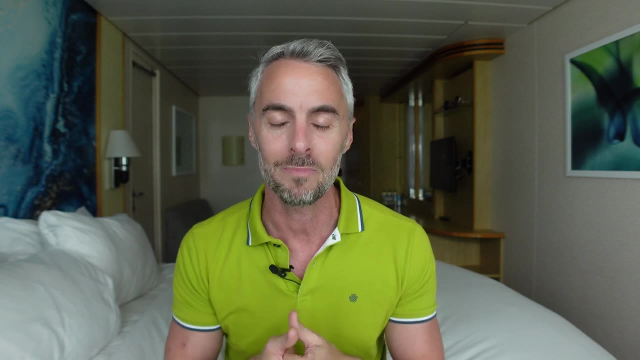 can throw at me at this point, But over in the Mediterranean they're pulling from a different pool of people because it's just cheaper to fly somebody from Europe to the Mediterranean than it is from the States over to the Mediterranean. You're also going to see that the music and the 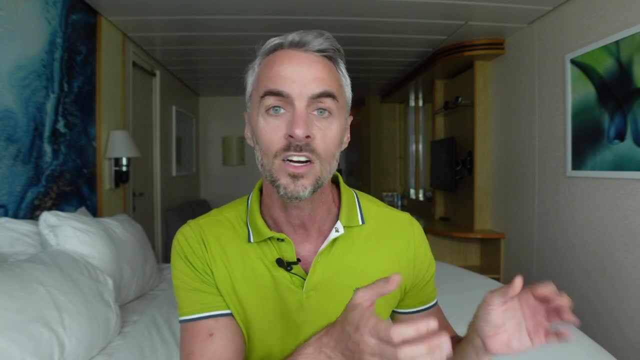 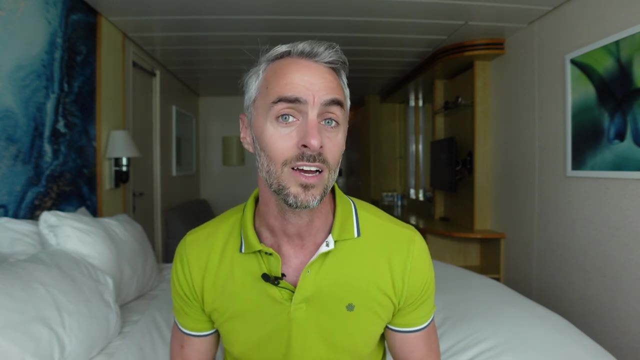 songs that they sing are going to be much more international. You're not going to hear only English spoken songs. You will absolutely hear probably two or three other languages that are going to be sung. I know we heard a lot of Spanish, as well as Italian songs. 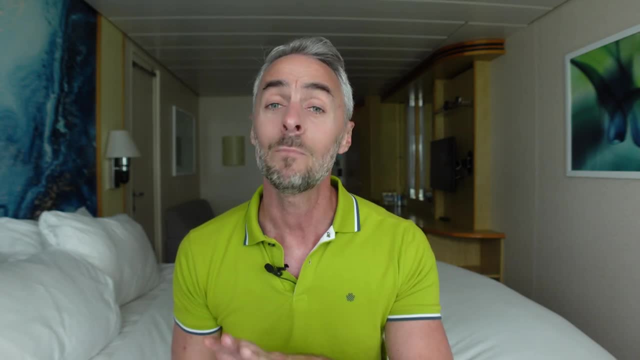 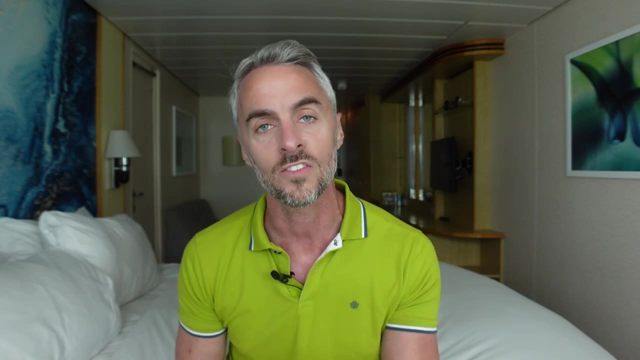 on our cruise, since we took off from Ravenna, Italy, But that was awesome. I personally didn't know all the songs, but from the people that were singing along I knew that they still were very popular in different cultures. All right, everybody, so I truly do hope that you are trying to get out. 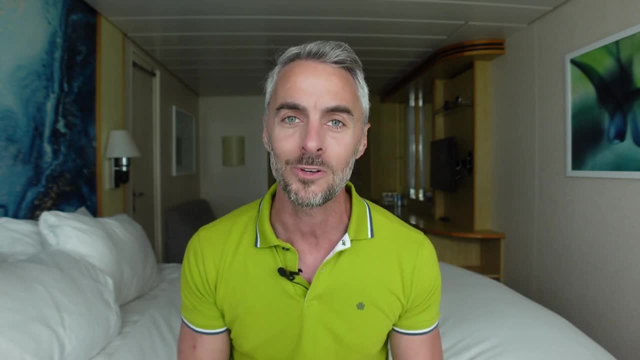 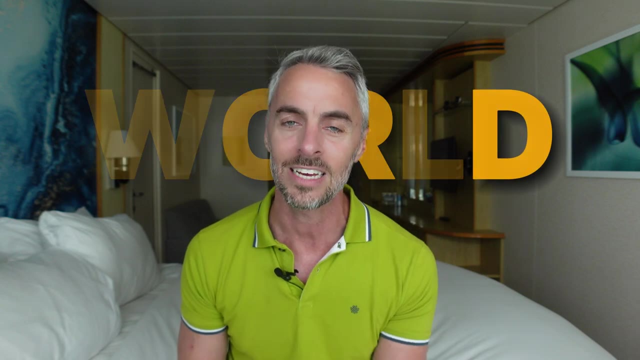 of the Caribbean. I think that the Caribbean is wonderful, but if you have the opportunity to experience more of the world, especially via cruise ship- one of the easiest ways to travel and see a lot of places at once- I hope you are taking advantage of that. 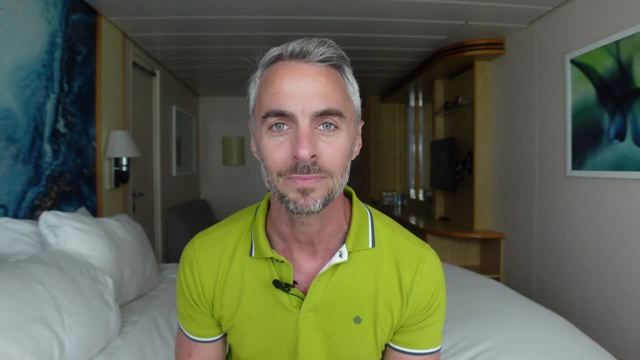 All right, everybody, this is Brandon, The Weekend Cruiser, hoping to see you on a weekend cruise soon. See you soon.